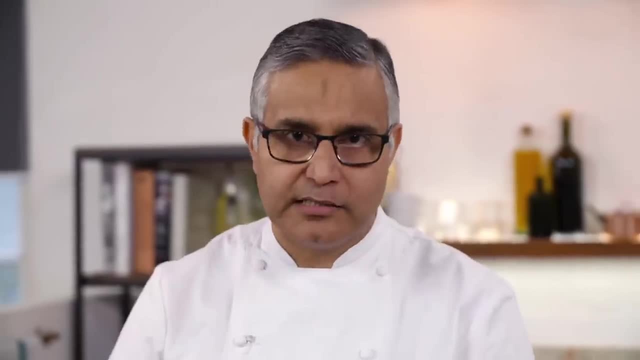 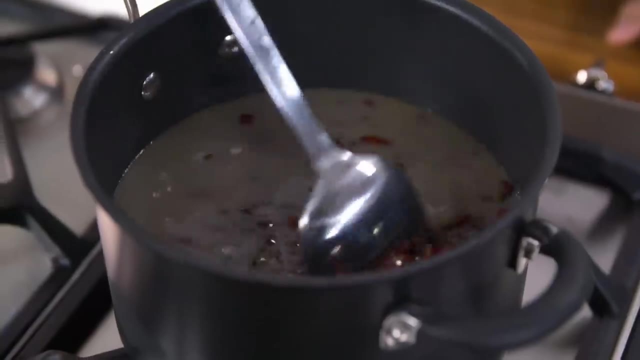 And I also prefer it like this. It'll take at least 90 minutes easily. I have beautiful memories around this pot of dal being brewed, stewed, in the house, And the whole house would linger with this, This beautiful nutty flavor of dal. 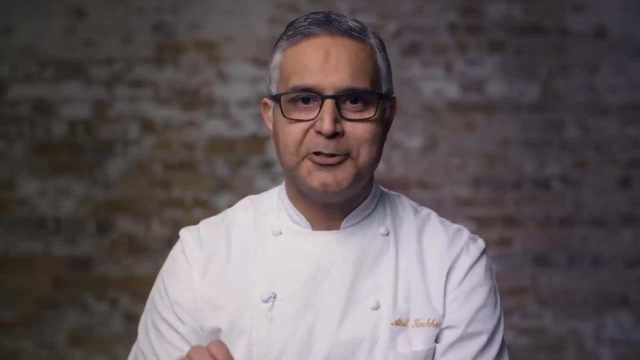 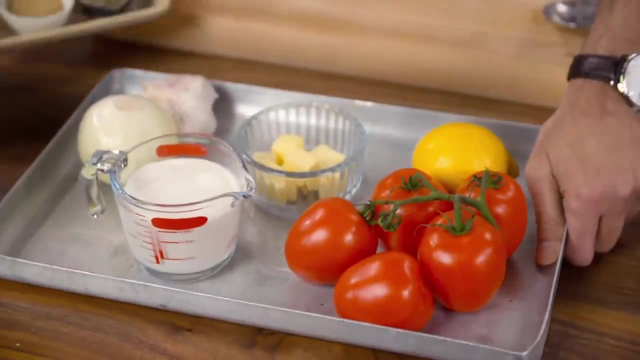 And wherever I was in the house I could smell that dal makhani is coming on the table tonight And I would salivate all day. I have to make seasoning, stroke masala to go into the dal, to make it dal makhani. 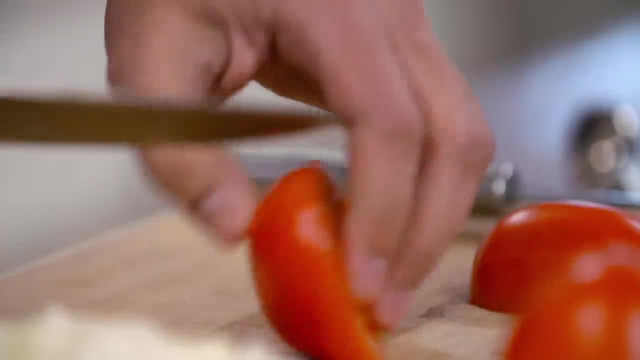 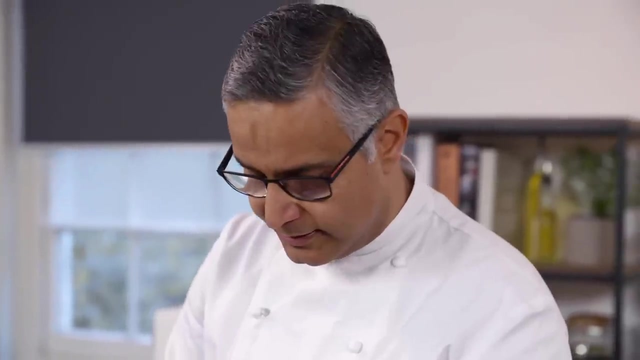 Everybody says that it's called dal makhani because the word makhan means butter in Hindi. It's true, there's a lot of butter in there, but it's called dal makhani because of its consistency, It's flavor, It's taste. 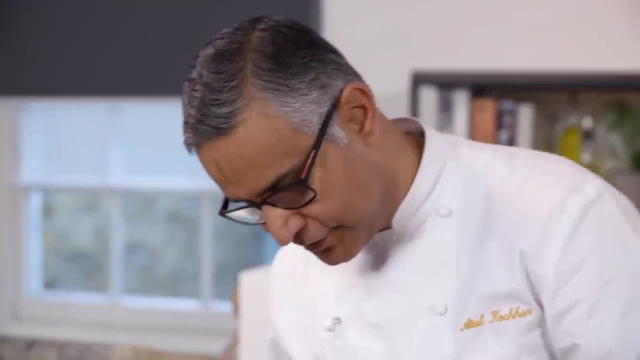 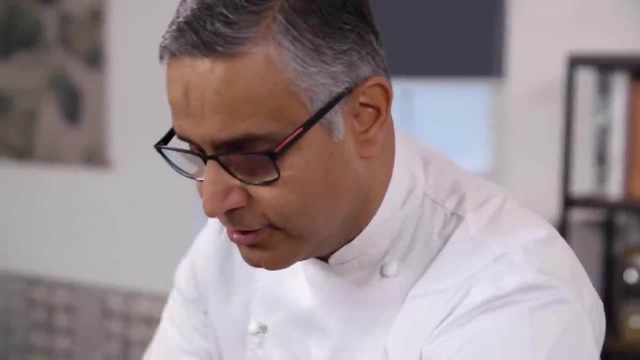 I still remember the day when I started cooking this with my mom first time. She would make me wash that lentil first for hours And then she would say, okay, now we need to put them for boiling, Chopping, peeling, scraping- all that was part of me growing up in my mom's kitchen. 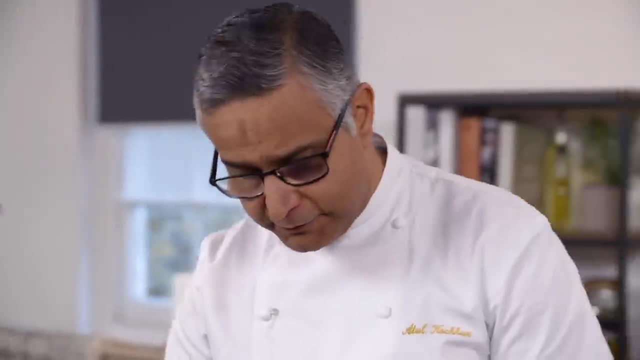 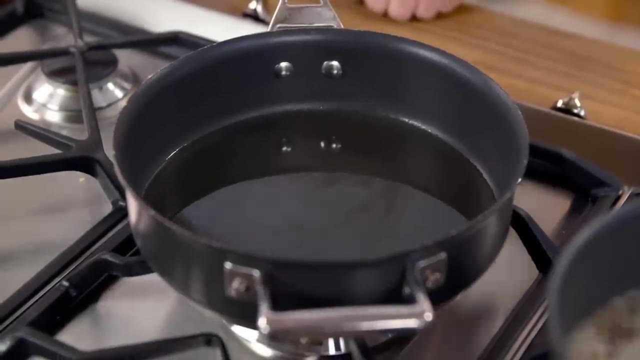 As a cook, my job is to extract the flavor of the essential oils in the spices into the dal, And that's what I do. I bring the oil to the right temperature, which is just below the smoking point, and then add the cumin or whichever spice I'm using, and it crackles immediately. 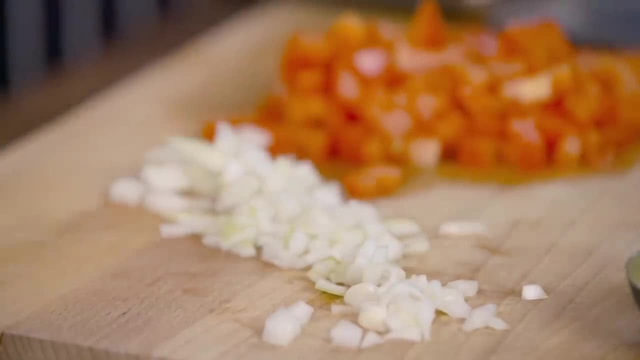 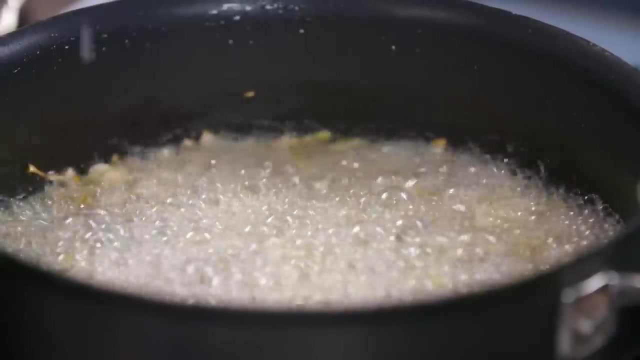 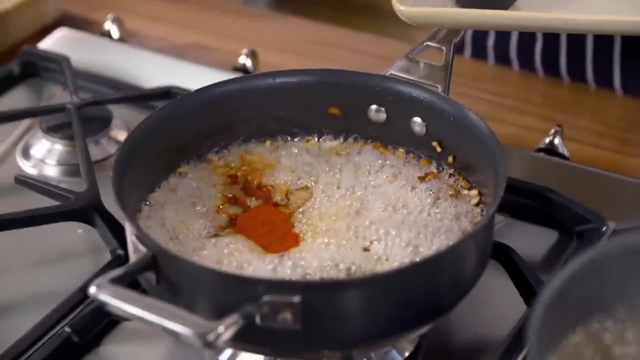 I'll add all the onions You've got to know, your onions to cook Indian food. Now, the powdered spices, coriander powder, the red chili powder. The powdered spices get burned very fast. Hurry up from here And then cook it through. 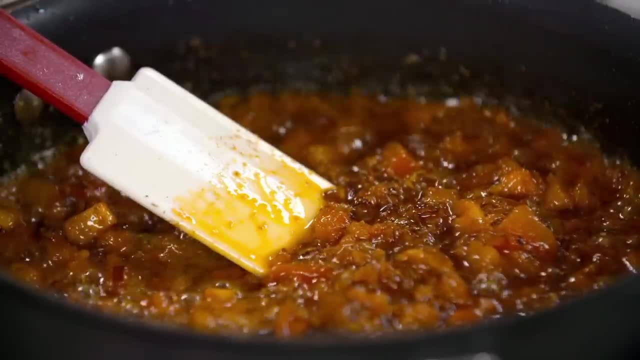 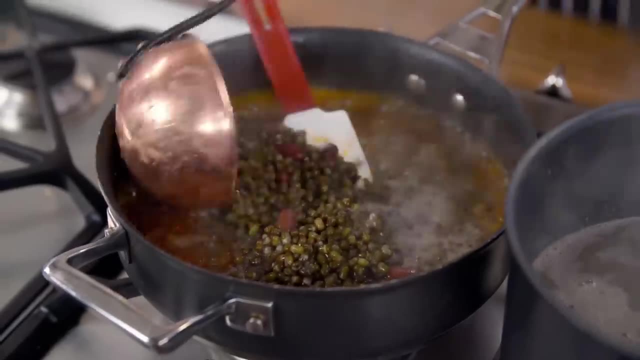 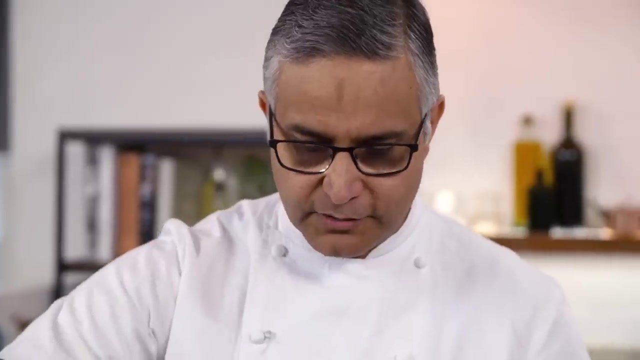 Okay, now the tomatoes kind of start disintegrating and that's the time I can start bringing in the lentil. You don't drain it because you need all that water in here. From here this takes half an hour to 45 minutes. 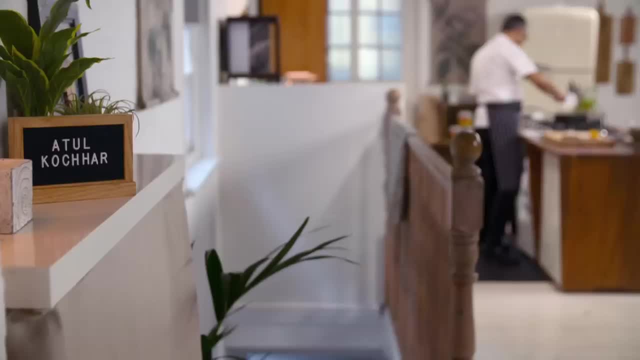 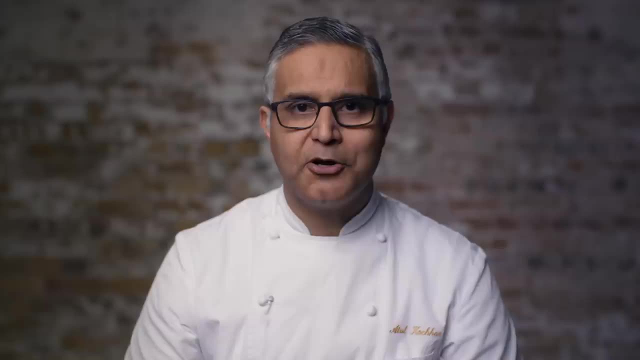 Being with my dad, being with my granddad, being with my mother, my siblings- they're doing great things. I think life was just so beautiful. We didn't have a lot in terms of economics, We didn't have a dining table at home.